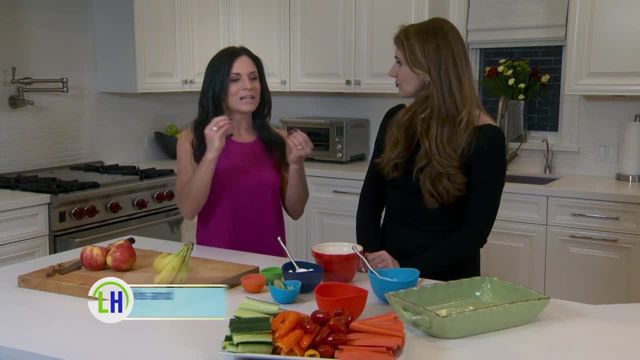 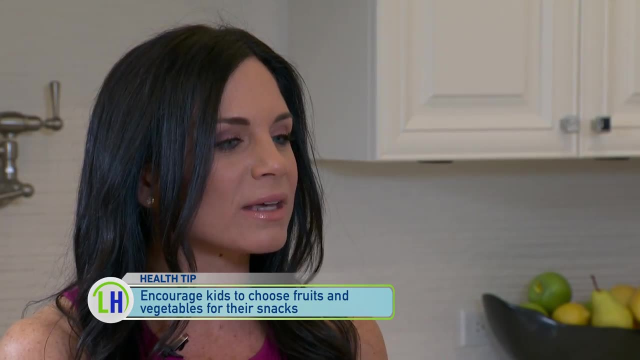 Rather than kind of sticking to the convenient things that are in a package, in a box, looking to our fridge first and trying to choose things like fresh fruits and veggies, choosing things that are vitamin-packed and fiber-filled so that also empty quickly that they can be ready. 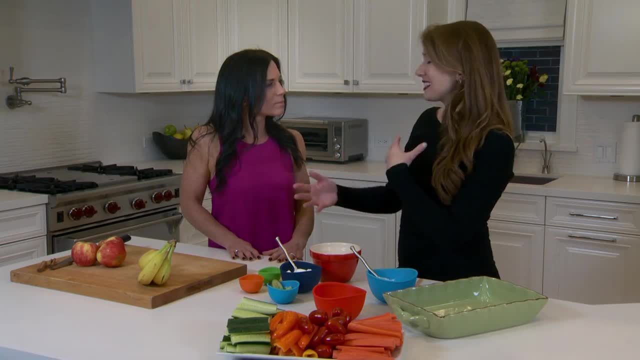 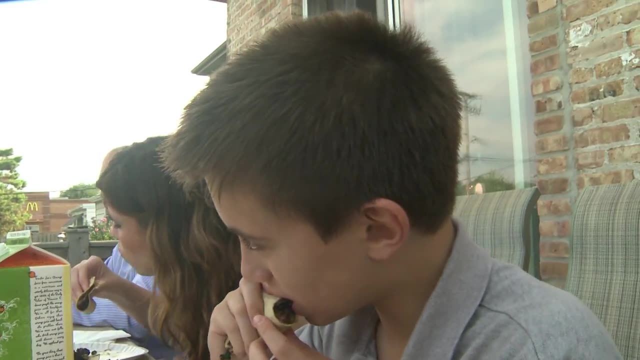 for the next meal. These habits and choices are also helpful to just getting good habits for adulthood as well, right, If we are establishing good habits in childhood, we will establish them in adulthood as well, And you have a few recipes for specific snacks. 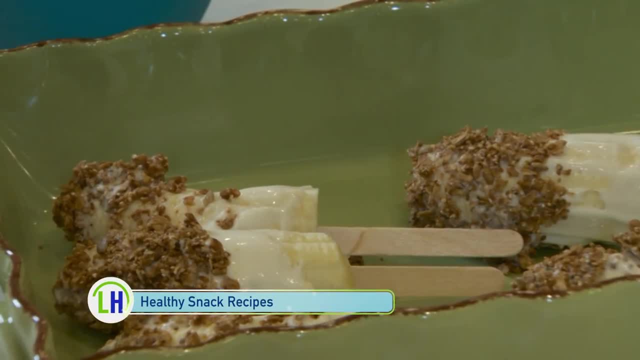 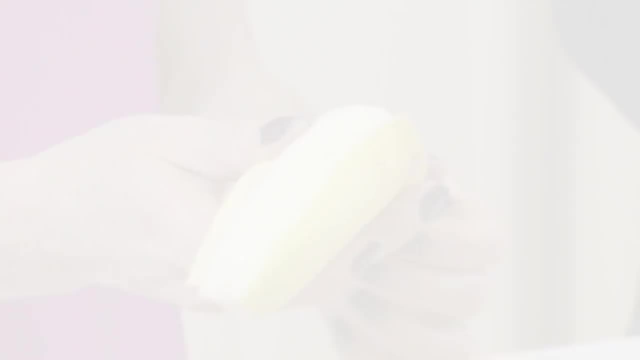 that you recommend. Let's get right into it. We're going to make banana pops, Greek yogurt, dip for veggies and apple chip. Okay, Let's get started with these banana pops. Sure, That sounds so fun. What I'm going to do is just take this banana. 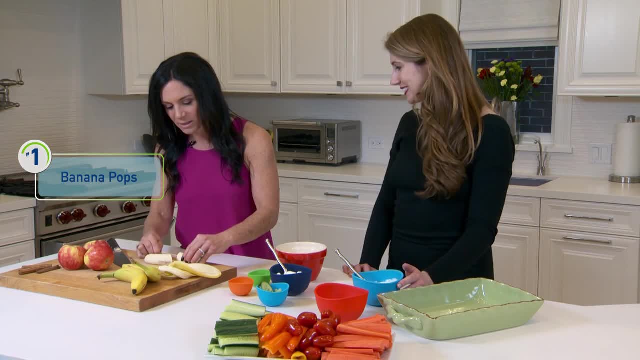 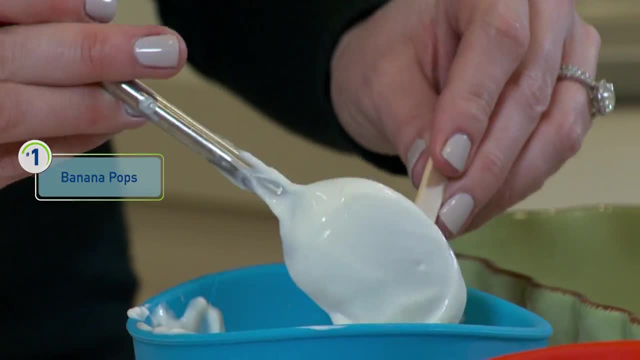 and slice it in half. I'm going to take a Popsicle stick and put it in the banana And I'm going to ask if you don't mind to dip that in some Greek yogurt. Then we're going to dip it in the banana. Okay, 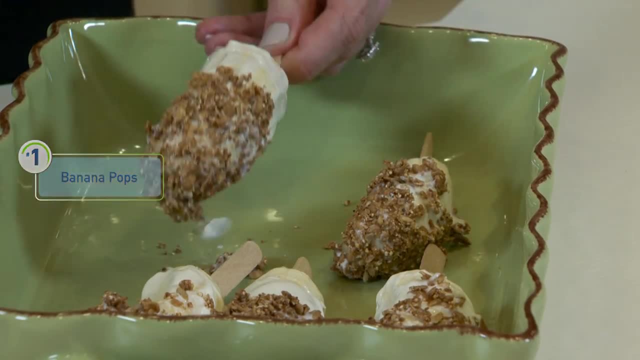 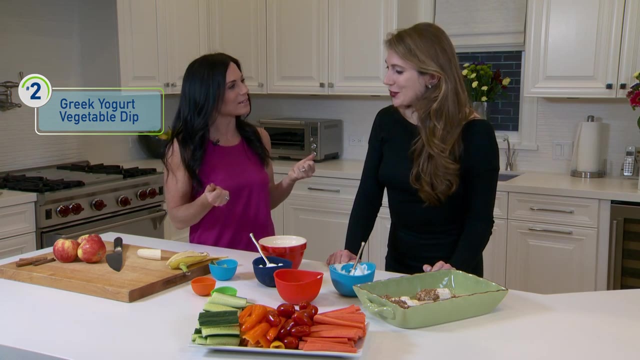 And dip it into the granola and just put it on that tray over there. Okay, What's snack number two? a dip Sure Veggies. by themselves, sometimes they're not that fun, And so trying to make them fun and exciting is one of my number one goals. 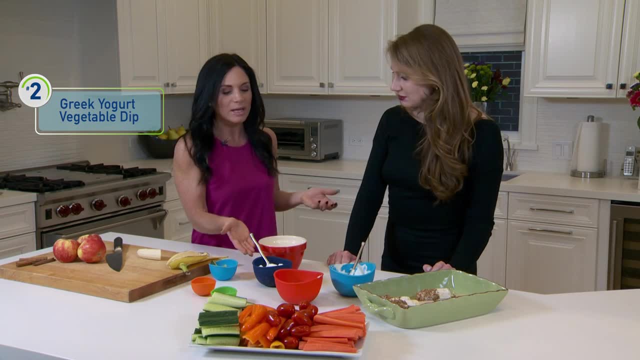 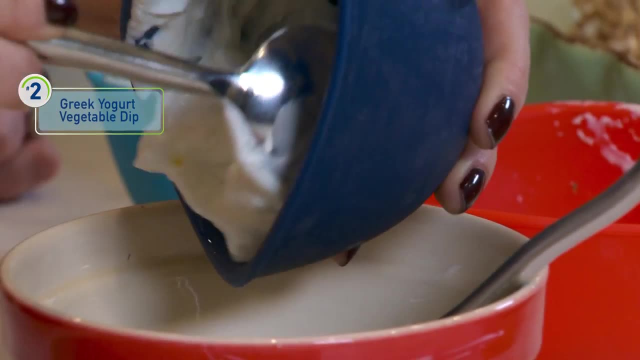 but also trying to put something valuable in our dip, And so I'm highlighting here Greek yogurt. Greek yogurt is calcium-filled, protein-filled, full of long-lasting nutrition, So we take Greek yogurt, plain Greek yogurt, making sure that it's fat-free. I take a cucumber and 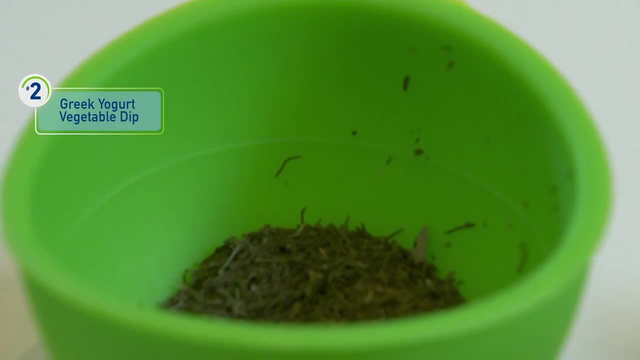 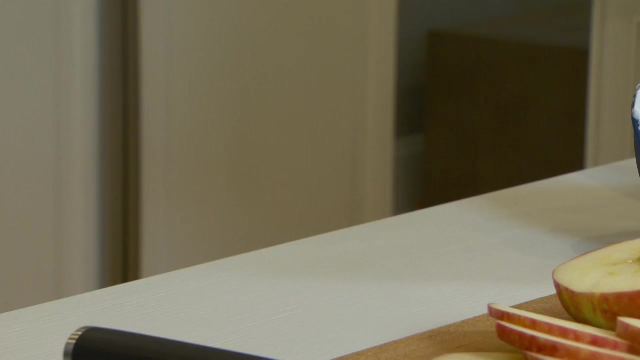 I shred it and we just plop that right in. You can use fresh or dry dill, Pop that in and then salt and pepper, So you mix this all together. We grabbed a big bowl to make our final healthy snack. 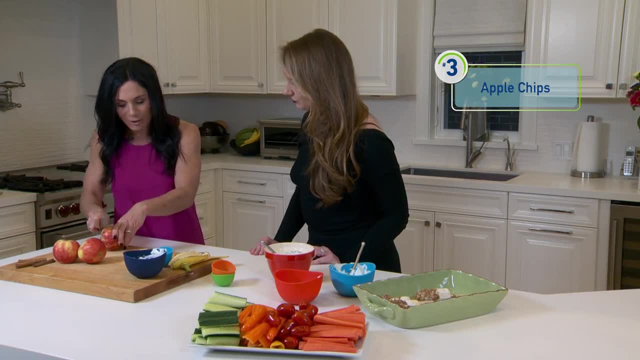 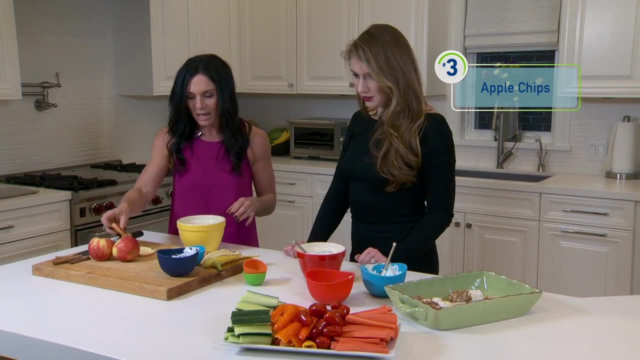 These are apple chips. So we take a fresh apple and we can carefully slice it into circles, And we're going to take this and toss it in with some cinnamon and a little bit of sugar. We set the apples out on a baking sheet to prep them for the oven, And then 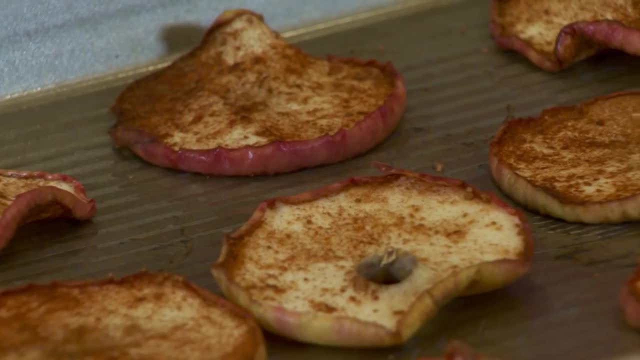 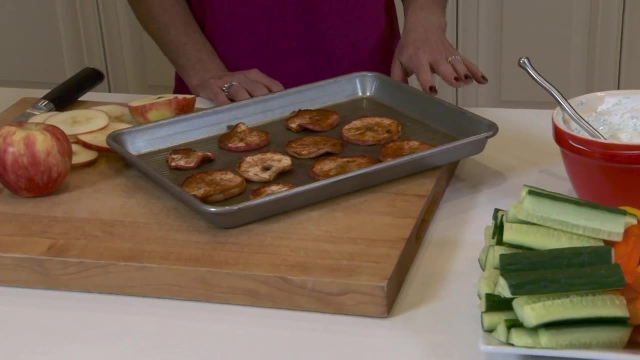 we're going to set our oven to 200 degrees and then place these in the oven for an hour. They were easy to prepare, easy cleanup. What's the bottom line when it comes to snacking? I think just trying to go for the fridge and get out of the pantry.